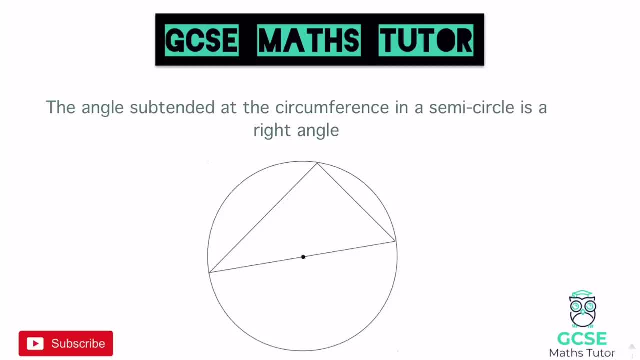 some nice examples on these. That way, obviously, when we do come to practice them in the next video, you can actually have a look at using those notes and actually applying them to specific questions. So for the first one that we're going to have a look at- and they're in no particular order, it just 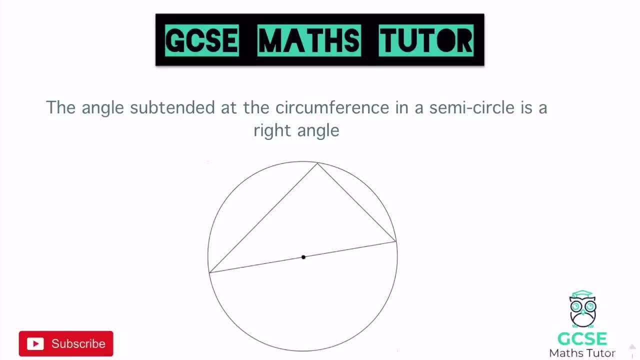 tends to be the way that I actually look at them. We're going to have a look at this circle theorem here. that says the angle subtended at the circumference in a semicircle is a right angle. Now, obviously, if you're not sure, this word here, subtended just means made, so it's just a fancy. 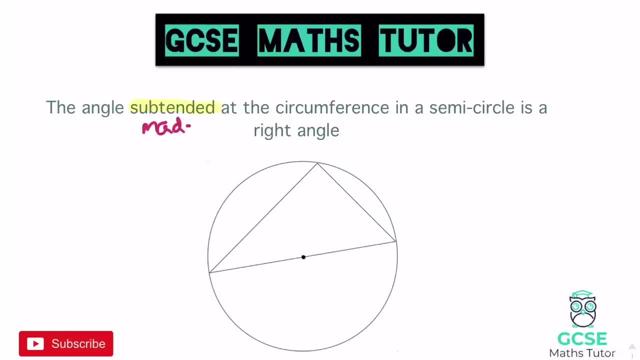 word for made, really, But the angle made at the circumference in a right, in a semicircle, is a right angle. Now, when we're looking for this circle theorem, in particular questions, what we're actually looking for is this line here, the diameter. Now, if there is ever a diameter in a question, chances are. 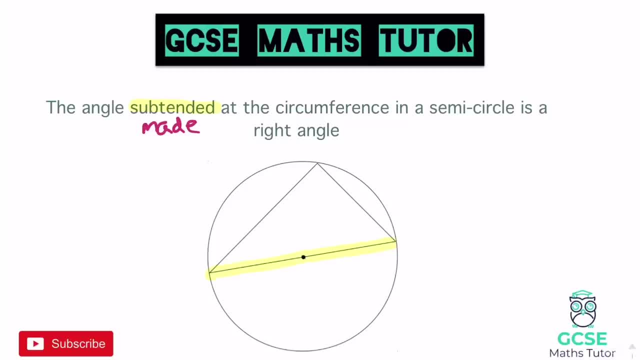 that there is a right angle at the circumference And obviously what this actually means, look, is from these two points: at the circumference, from the diameter, if we follow the lines up- and I'm going to draw them in- if you follow the lines up to the circumference here and from the other point coming, 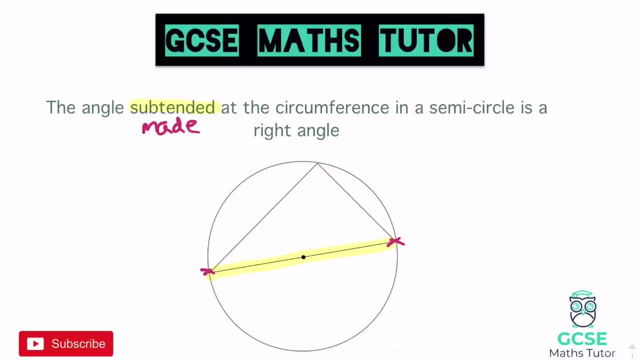 up to here. that angle there forms a right angle. OK, so if I get rid of that, this angle here is our right angle. Again, it doesn't matter where those two lines meet at any point on the circumference, as long as they come from the ends of the diameters at the circumference. 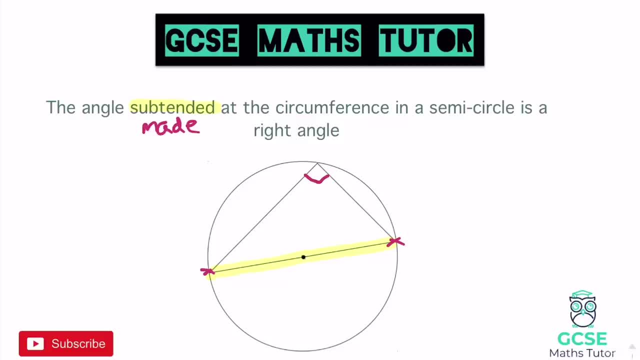 They form a right angle up there. OK, obviously this is usually involved in other questions, but that is our first circle theorem, And a little tip for that is: always look for a diameter, and if you see a diameter in a question, you're probably looking for a right angle somewhere. There we go. let's look at our next circle theorem. 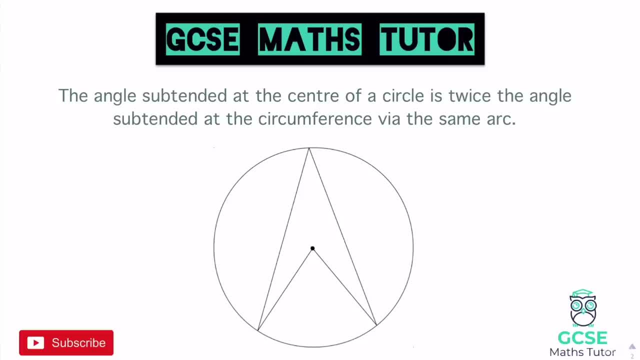 OK, so this circle theorem can be shown in lots of different ways, but it's typically known by this sort of arrow shape and it says the angle subtended or angle made at the centre of a circle is twice the angle subtended or made at the circumference via the same arc. Again, we can obviously split this. 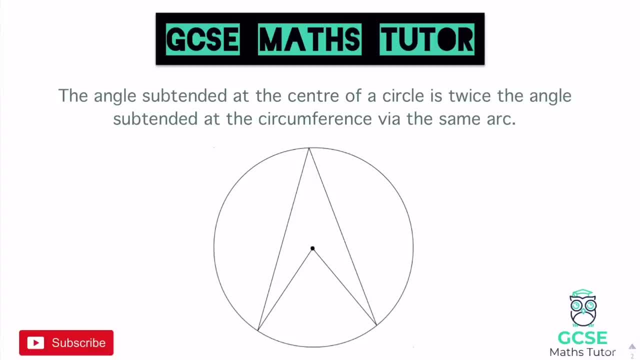 in reverse, we could say: the angle at the centre is half. sorry, the angle at the circumference is half the angle at the centre, but obviously it doesn't really matter either way. Now, this is quite the nice way of actually seeing it, but basically we're looking for angles that are made at the centre. 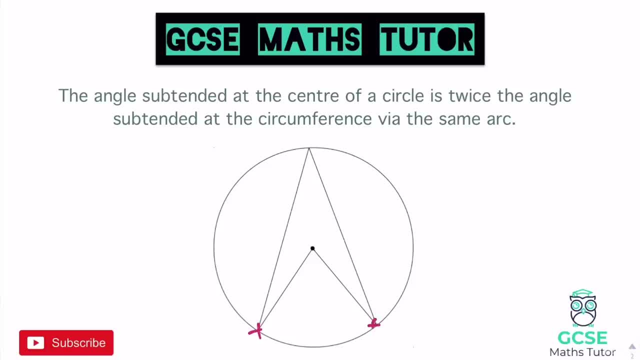 from these points here. So if you ever have angles made at the centre- and I do normally sort of trace along this with a highlighter- I think OK, well, this makes an angle at the centre. and then I have a look: does do those two points make an angle anywhere else? and if we trace from the centre to the centre, 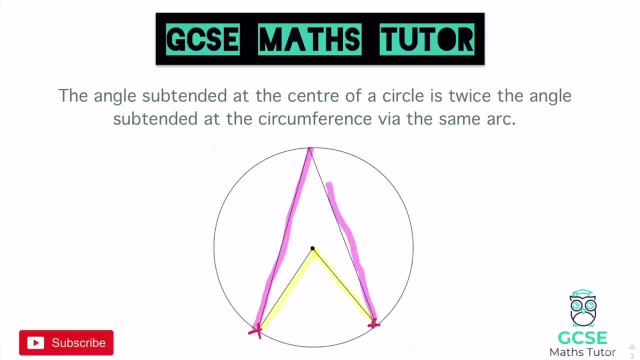 from those points up to the circumference there. it does actually make this angle here at the top. So obviously that's what we're looking for when we're looking at these questions. we're looking: is there an angle made at the centre? and if there is an angle made at the centre, do those same two points on the 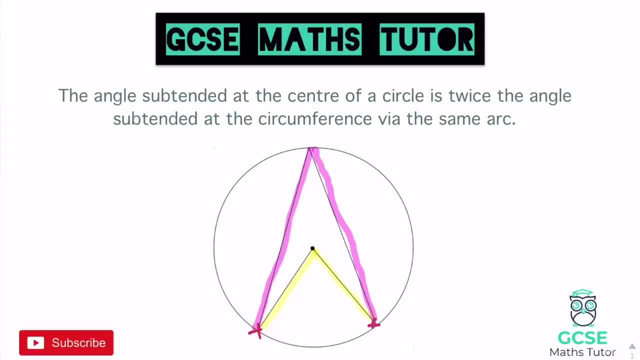 circumference, or from those same two points on that little arc there make an angle anywhere at the circumference. So if we actually have a look at this, look, if I was to allocate a number, I'm going to pick a nice, easy one here. but let's imagine this one is 80 degrees. quite nice, and simply this one up. 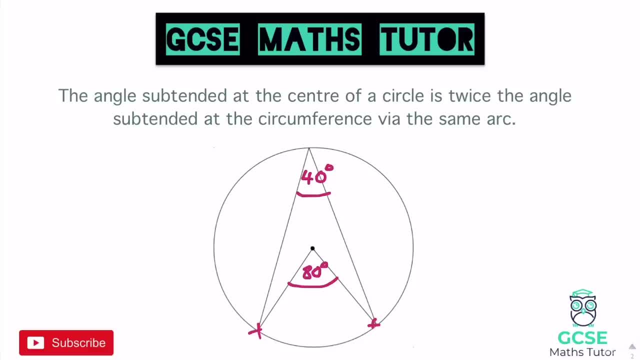 here is half of that: 40 degrees, And likewise the other way. if we have the angle at the circumference, we would be able to double that to get the angle at the centre. So when you're looking for this circle theorem, obviously just make sure you're having a look for angles that are made at the centre. 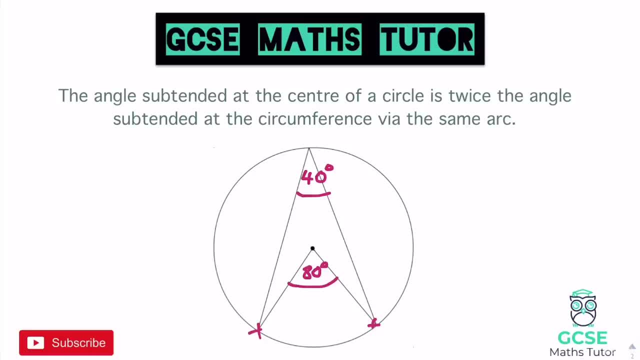 and then just see, from those two points can you trace your fingers or, using a highlighter, can you find an angle made at the circumference as well. So that's our second circle theorem rule there. but you do need to bear in mind that obviously this actually can be shown in lots of 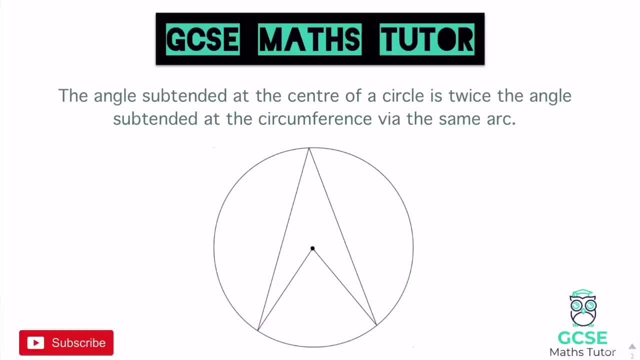 different ways and there's a couple of quite horrible ways that it can be viewed sometimes. So I'm going to go over this diagram. but if I was to say, have these angles here at the circumference, I could have the lines also. I'm going to do this in a different colour, going off at an angle that doesn't make this sort of. 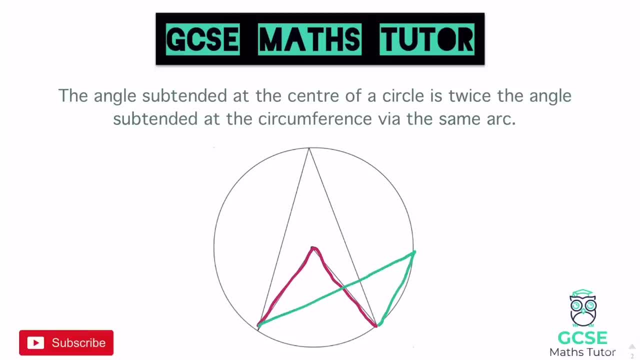 arrowhead shape, so I could actually bring it all the way up to here and bring it down there as well, And that would obviously still have the same same circle theorem here, but obviously it's not quite as easy to see. it doesn't make this nice arrowhead. 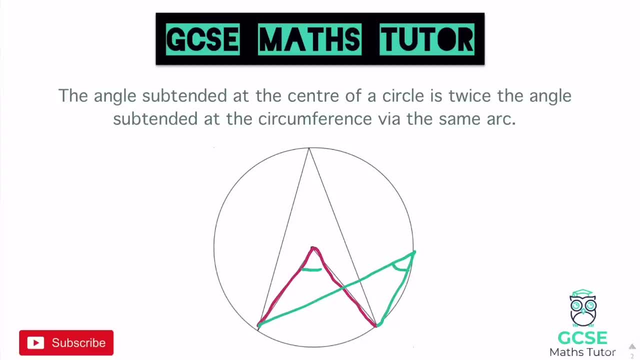 but this angle here is double this angle here. OK, so it's just that they can be seen in a couple of different ways and again, always just try and trace your- you know your finger or your highlighter up Those lines. so here's the angle at the centre and obviously from those same two points you could then find this angle over here. 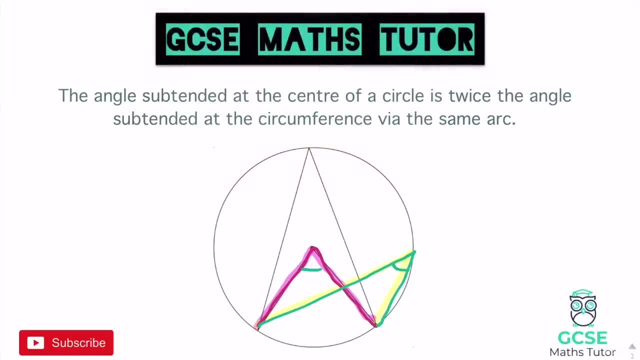 OK, but it's not the nicest when it is obviously pointing off in a bit of a strange direction, but just another way that you can actually see this circle theorem and something to be thinking about moving forward. OK, but there's that second circle theorem. let's have a look at our next one. 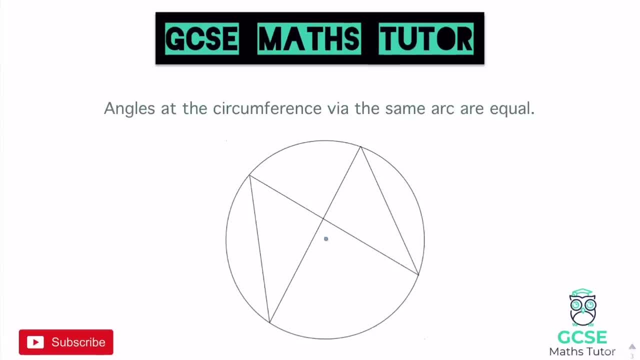 OK, so for our next circle theorem. it's: angles at the circumference via the same arc are equal. Also, sometimes, you know the circle theorem rule, for this is sometimes said: as angles in the same segment are equal, It doesn't matter which one you use. 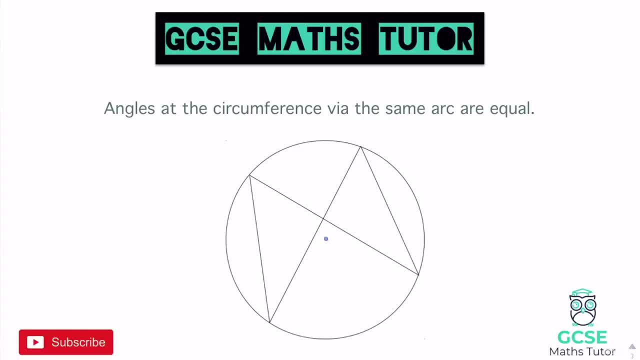 Here, but it's just about looking at the ones that we're actually going to find. Now, again, we've got angles that are being made at the circumference from the same arc. So if I pick these two points on this little arc here, here and here and again, we can trace our fingers or a highlighter up to the angles at the 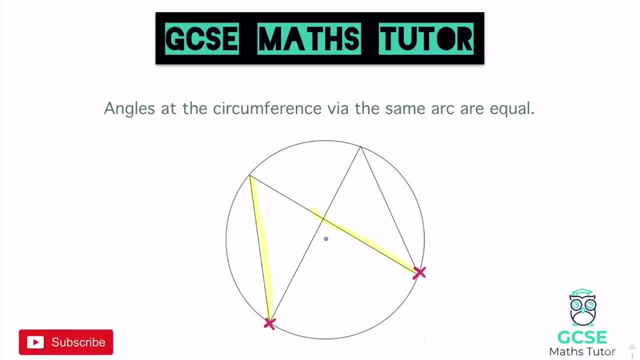 circumference. So from those two points, look, it makes this angle up here. and if I switch colours, if I go from those same two points, it also makes this angle just up here. There we go, So it makes these two angles just here. It's sometimes referred to as the bow tie. 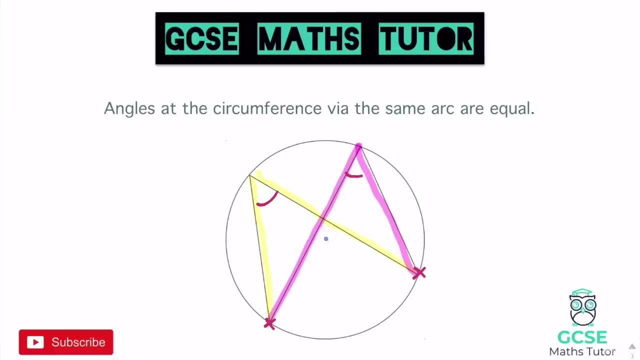 Circle theorem as well, because it makes this little bow tie shape as a little way of remembering it. It makes those two angles there. So if we had some numbers in there- and I get rid of this- let's imagine it says that this angle is 30.. 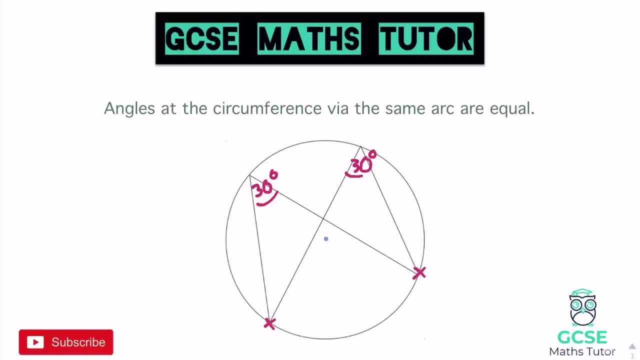 I would also be able to say that this angle here is 30 as well. OK, and that's those two angles, but this I can also be viewed upside down, because obviously I've viewed it in a specific way. Now, if I get rid of all of this and get rid of these two points, I could also look at these two here. 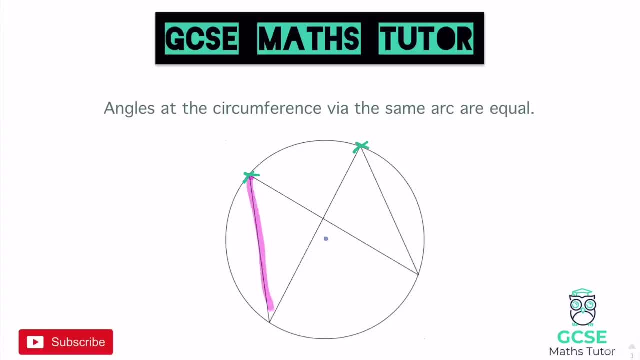 There we go. And again I could follow that same process Coming down from those two points. it creates this angle at the bottom and if I switch colours coming down here, there we go. It also makes these angles down here, So also these are going to be equal as well. 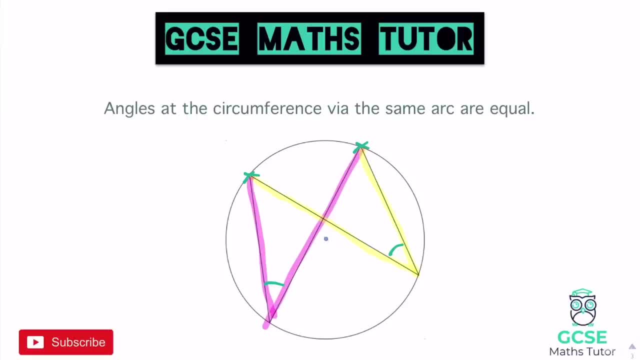 So again, if we, if one of those was 30 or 40, the other one would be 30 or 40 as well. So just obviously, thinking about that, they can be viewed upside down and thinking about those angle rules within this sort of circle theorem here. 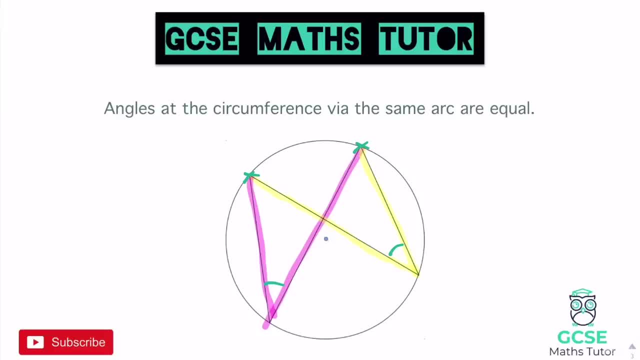 But again you're looking for, just like on the last one, once you've got two angles, or I mean two angles that are made from those points on the arc. They could be at the centre, They could both be at the circumference, And there's two different circle theorems depending on where those angles are made. 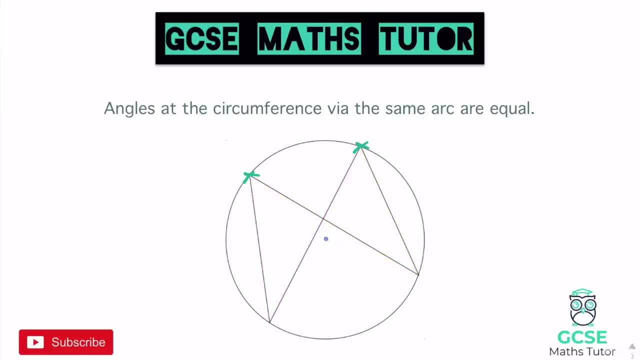 OK, and obviously also thinking about this, you've also got another angle in here which you could be thinking about as well, and that's these two. And these two angles are vertically opposite as well, so they're also going to be equal. So not really part of the circle theorem, but obviously just something to be thinking about in terms of our angle rules when you are faced with this sort of circle theorem and particular angles in these sorts of questions. 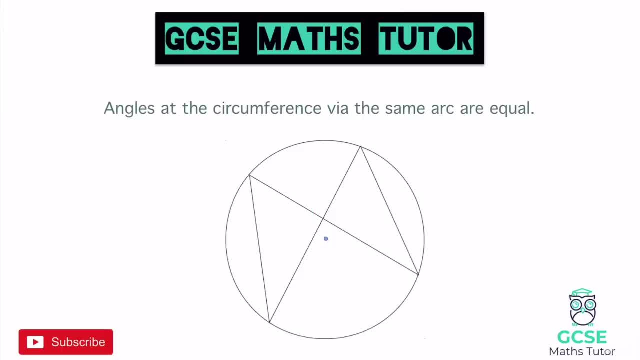 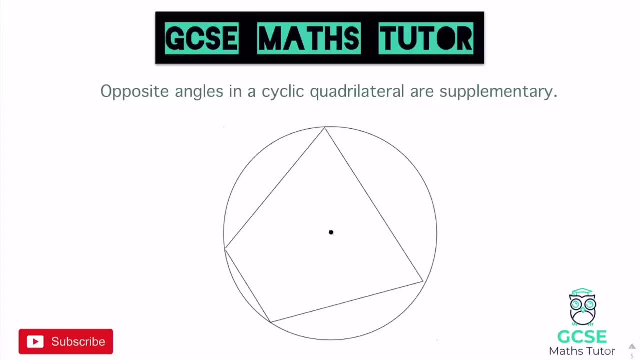 OK, but there we go. There's our third circle theorem, and we're going to have a look at another one. OK, So our next circle theorem is: opposite angles in a cyclic quadrilateral are supplementary, And that word supplementary just means they equal 180 degrees. 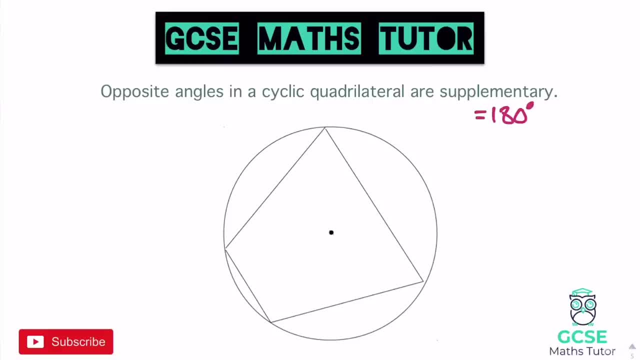 So opposite angles add up to or sum to, 180 degrees, and that's that word supplementary there. So opposite angles refer to these. So if I pick one of these angles here, the one opposite that, if I was to draw a line out, would go opposite over to this one. 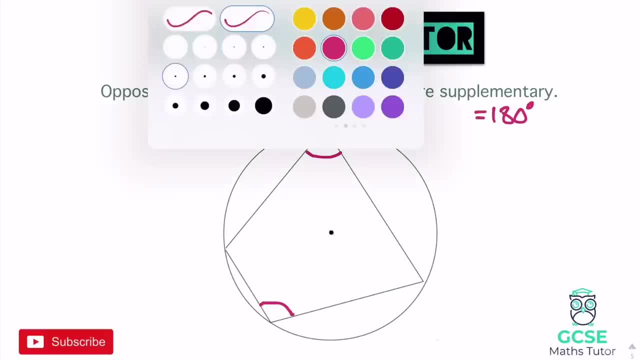 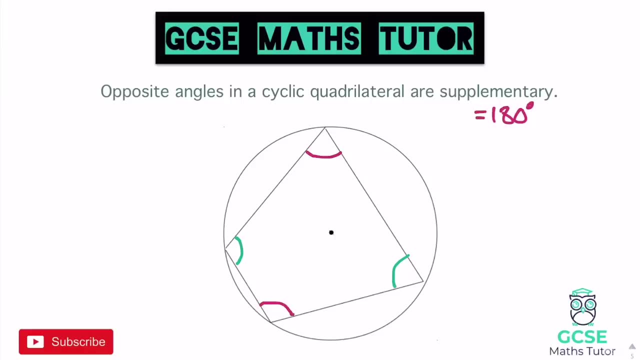 So these two angles here add up to 180.. Likewise with the opposite two as well. if we've got this angle here that's opposite to this one over here, So these two also add up to 180 as well. Now, what is really important with this is it does have to be a cyclic quadrilateral, and that means that the four vertices of that quadrilateral join up on the circumference of the circle. 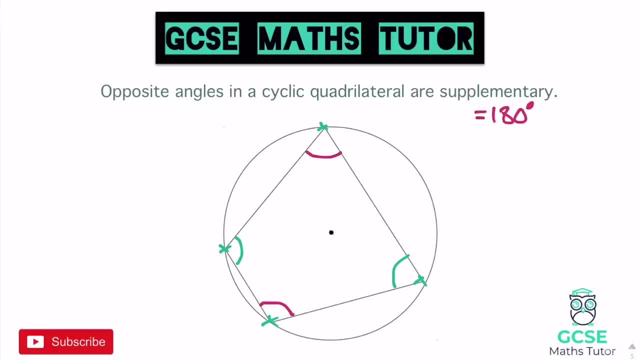 OK, So it can't just be any quadrilateral, It can't be. Let's just have a think about how I could draw one of these. So let's imagine we've got three points there and the last one. There we go. 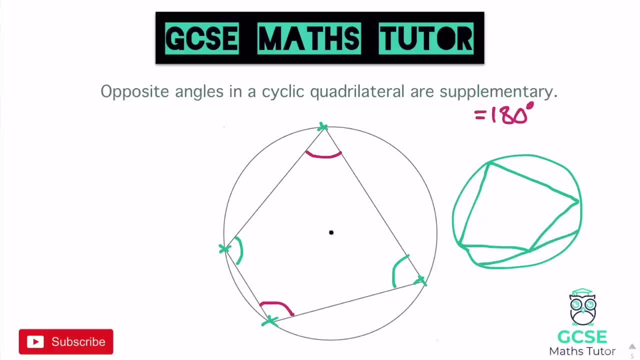 It doesn't connect. Maybe there's another line in there or something like that. OK, That would not be a cyclic quadrilateral, because all those vertices don't join at the circumference. So it's got to be very specific here in terms of the actual way the quadrilateral is drawn. 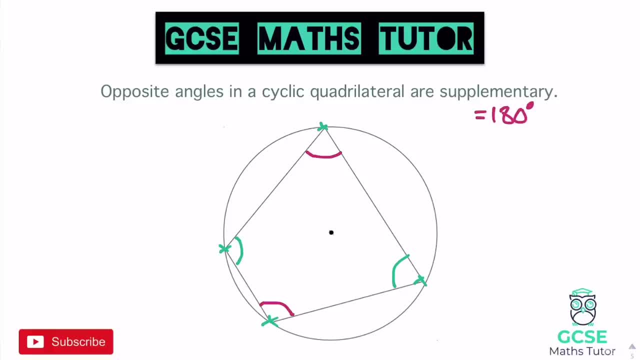 It doesn't have to be a cyclic quadrilateral, But those opposite angles there add up to 180.. So obviously, if this one here was 50, which obviously isn't because it's bigger than 90 there, But if it was the opposite angle would be 130.. 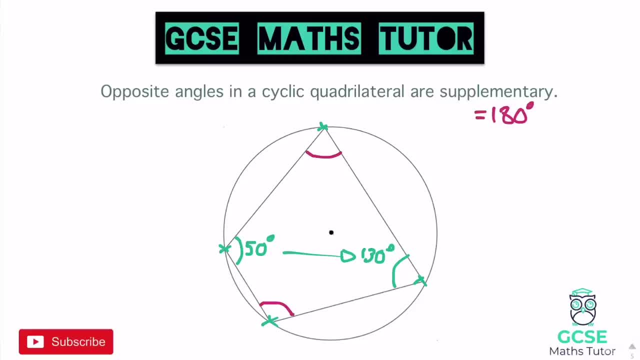 Probably should have done that any other way around, really to make it look a bit more realistic. But that one. if the numbers said that that was 50 and the opposite one would be 130.. OK, Likewise with the top two there. If I allocated one number to one, I'd be able to find the other one by subtracting it from 180. 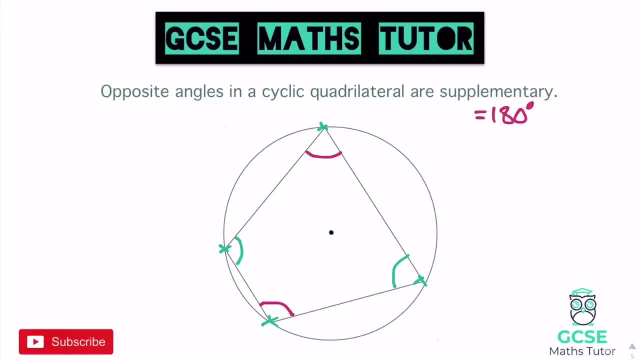 But there we go. That is our cyclic quadrilateral. Again, just thinking about how you would actually look for one of these. Obviously you're looking for a quadrilateral within a circle, But just thinking about the fact that those points do all have to be on the circumference there. 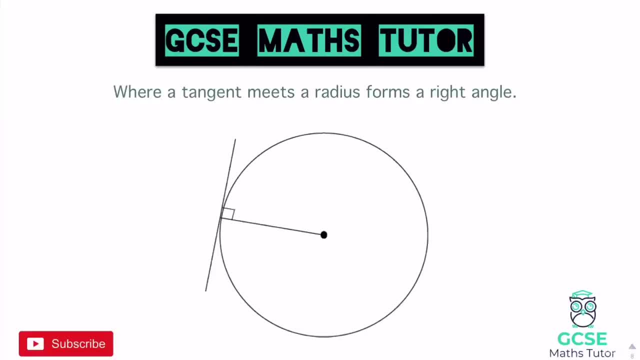 Let's have a look at our next circle theorem. OK, So for our next circle theorem, it's where a tangent meets a radius forms a right angle. So I've drawn the little right angle in here, But we've got a tangent which is obviously a line which just touches one point on the outside or on the circumference of the circle. 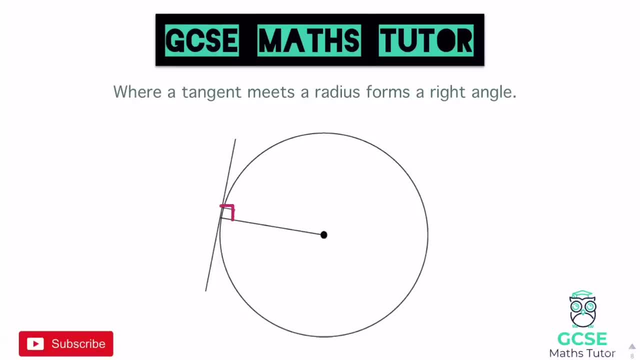 And at that point, there where it meets, the radius forms a right angle. And it's always good, just whenever you have a question like this and you see a tangent and you can see a radius, just to draw that right angle in. But there we go. 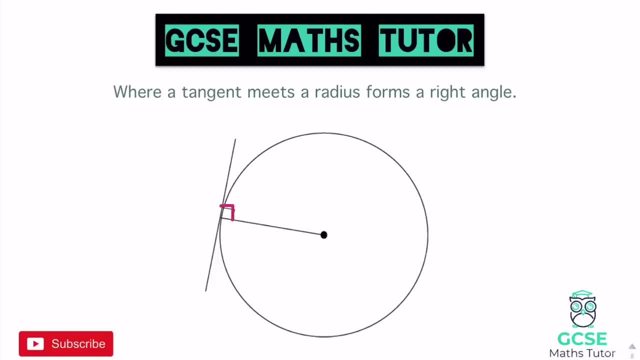 That's quite a nice easy circle theorem there It's just looking at. obviously, if there is a tangent involved in the question, chances are there's going to be a right angle somewhere And that right angle may be split up via other lines, But there is going to be a right angle there where those two lines meet. 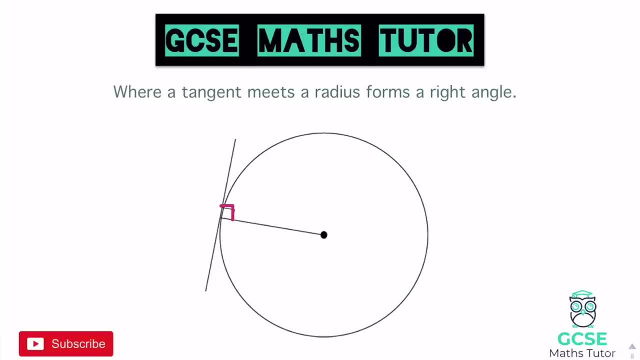 And it's where the radius meets the tangent. OK, So that's just a nice little quick circle theorem there when we're looking at tangents. There is one other circle theorem really, where we're looking at tangents. We're going to have a look at that one now. 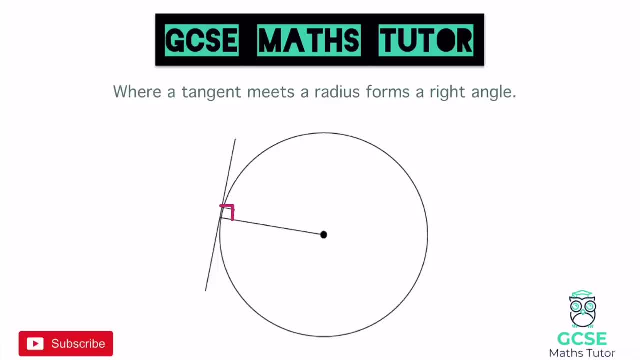 But this is our key one here, really, where we have got that radius meeting the tangent and forming that right angle, And on to our next one. So for our next circle theorem looking at tangents, it's this one here and it's where two tangents meet at equal length. 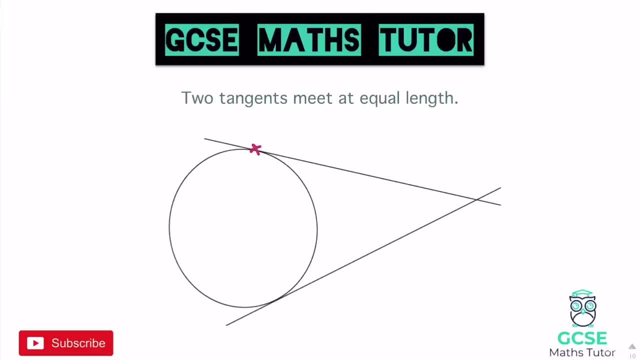 So all that means is from this point here to this point. here is the same length as this point, here again to that point at the end there, if I go over it again. So these two lines here are the same length, OK, And that's going to. 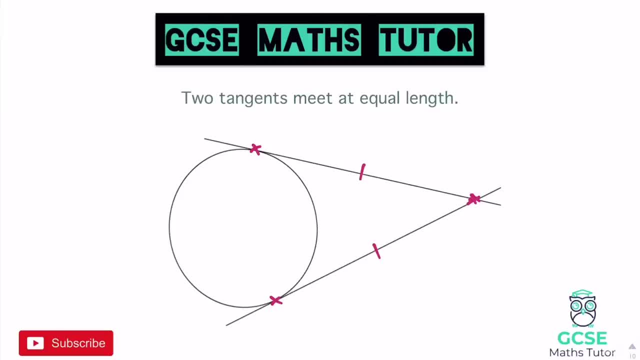 So quite unique questions when these do come up. but it's a good one, obviously, to make sure that you do know just when we're looking at these sorts of questions here. Sometimes there's obviously going to be a lot more lines in there. It could be that. 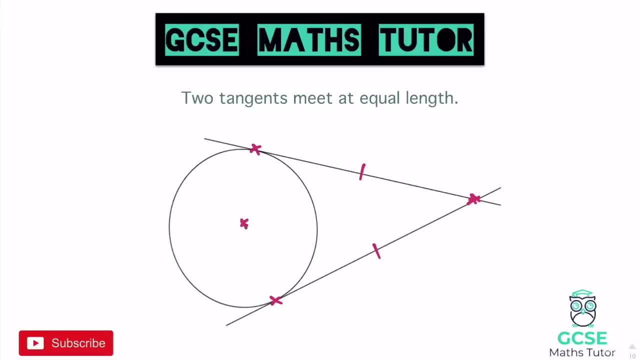 Here we go. If I try and draw the centre in, It could be that we've got some radiuses connecting down And maybe we've got some triangles to look at. Sometimes you'll see this line sort of drawn in like this And it forms these sort of right angle triangles. 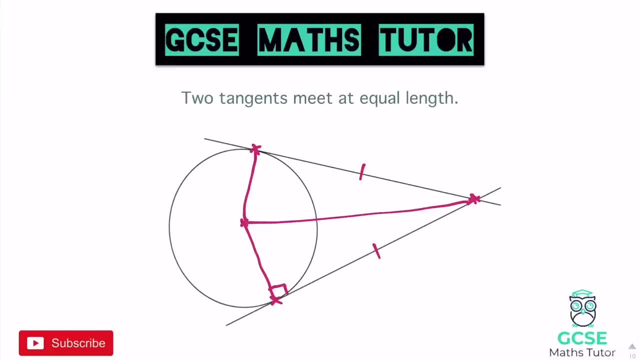 And we can sort of test all different sorts of things like Pythagoras and Sokoto within those as well. But that's just one other thing to be aware of where two tangents meeting at equal length. I'm going to have a look at our last circle theorem to finish this off. 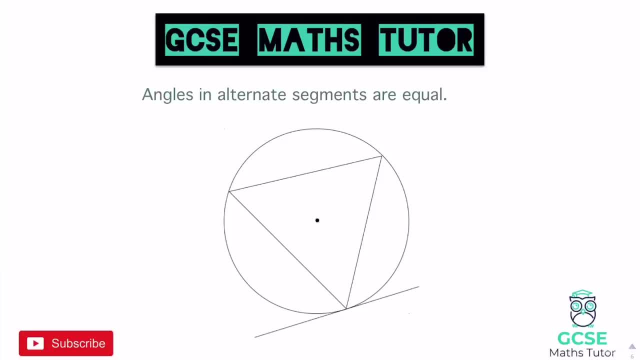 OK, So for our last circle theorem, we've got angles in alternate segments are equal And it's where we've got a triangle within a circle. We should really call it like a cyclic triangle or something, because these triangles do have to meet at the points of the circumference. 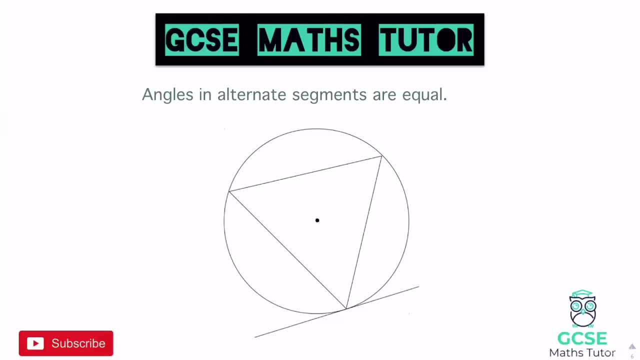 And we've also got a tangent down the bottom there. So where this tangent meets the triangle, it forms an angle on either side. So what I mean by that is: we've got this angle here. That's not drawn that in very well, We've got this. 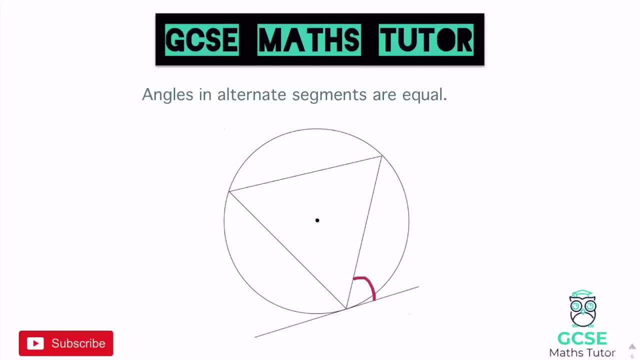 We've got this angle here And that is equal to what we call the alternate segment angle. So if we go through the triangle, Let's have a look. Imagine we walk into that angle and up the line of the triangle And it forms this angle just up here. 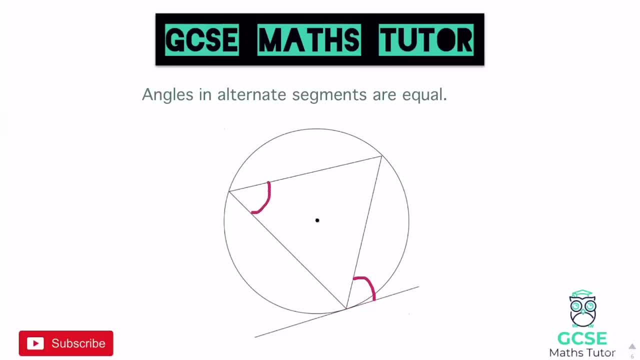 Now that angle there is equal to that one down the bottom And these are our alternate segments. OK, And they are equal angles. Now we also have one on the other side. We've got this one on the left, And if we imagine walking into that angle from the left here, 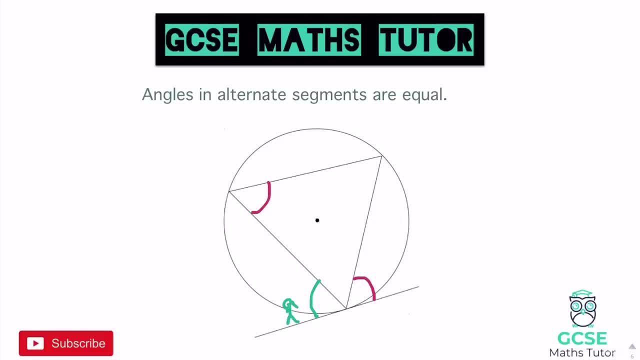 It seems a bit strange, but it can sometimes help to find it. If we imagine just sort of walking through the angle and up the first line of the triangle, Again it forms this angle up here And those two angles are equal. OK, And that is our alternate segment theorem here. 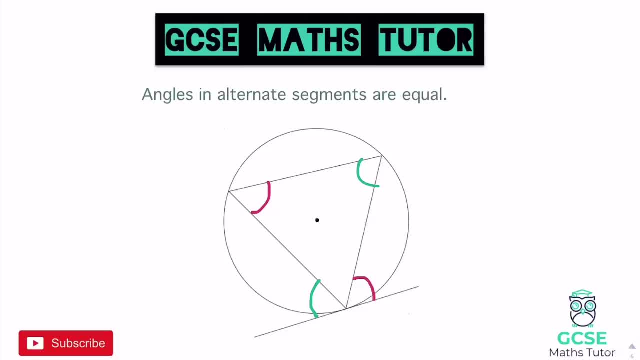 It's normally one of the not so nice ones to spot sometimes, But it's just where a triangle there meets a tangent And forms these alternate segment angles there. OK, So that's our last circle theorem, If you do want to have a look at actually understanding how these are formed. 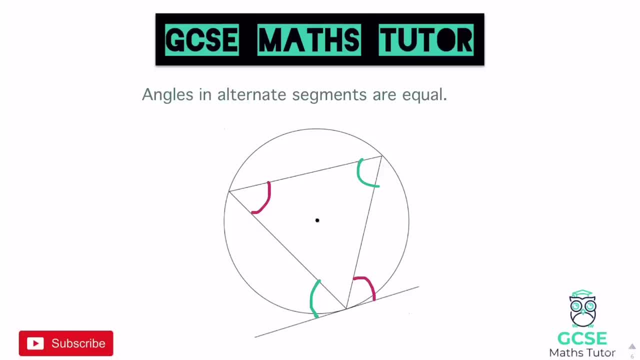 And the proof behind them. I'll link the video for that in the description So you can have a look at actually proving these angles And showing that they're equal using algebra. But these are all the circle theorems that you need to actually make sure that you know. 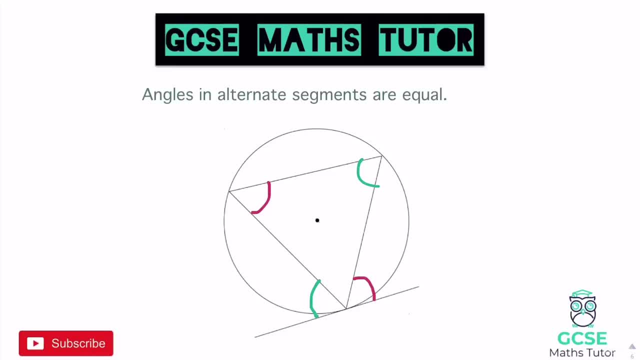 You're happy with them. You're happy to write down these descriptions Because the language is very important. A lot of these sorts of questions were asked for your reasoning, So you'll have to give the proper language behind these circle theorems. 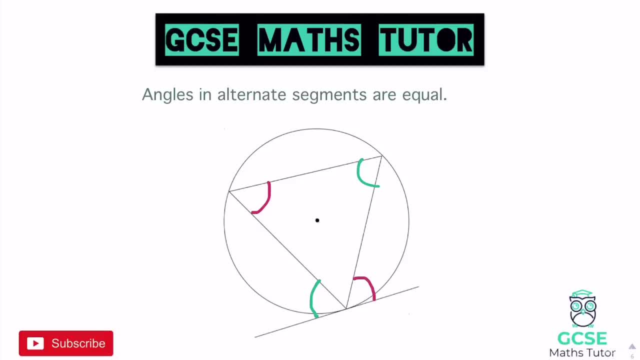 As well as actually apply them. So make sure that you've written them all down. Go back to the start of the video. if you haven't already, Make some notes on them, Obviously. make some nice, clear examples From where I've talked through them. 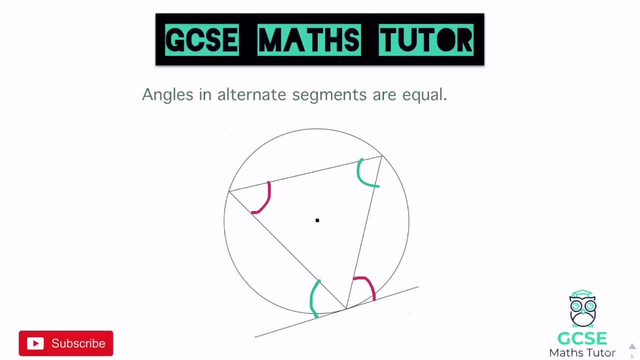 And then in the next video We're going to have a look at actually applying these to some particular questions. But in that video I am going to assume that you know these circle theorems. You're happy to sort of repeat them.